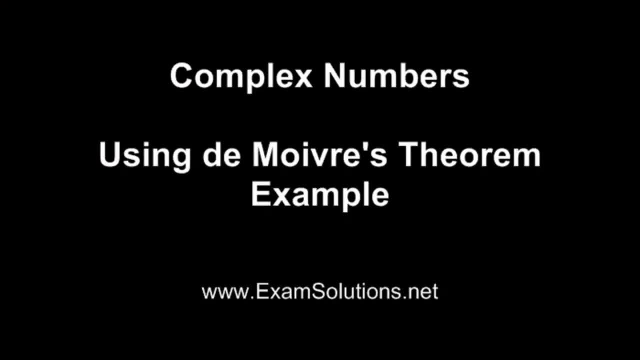 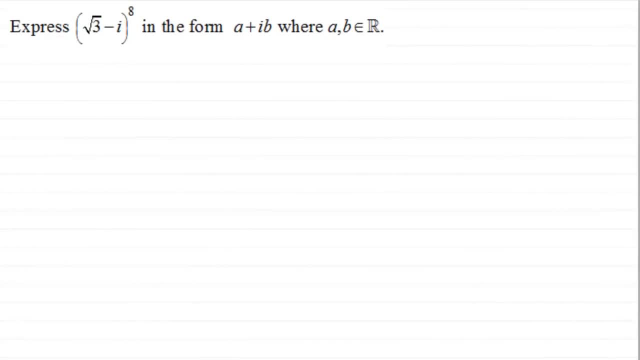 Hi. now I've got another example here that you might like to try. It's based on using DeMarva's theorem. What we've got to do is express root 3 minus i, all to the power 8 in the form a plus ib, where a and b are real numbers. 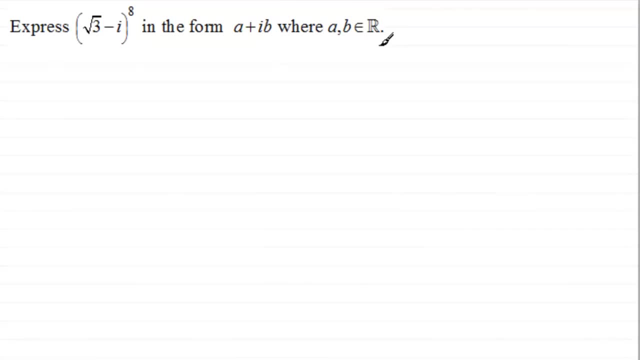 So if you'd like to give this a try, just pause the video, come back when ready and you can check your work solution with mine. Okay, welcome back if you had a go. Well, first of all, what I'd want to do is define z, a complex number z. 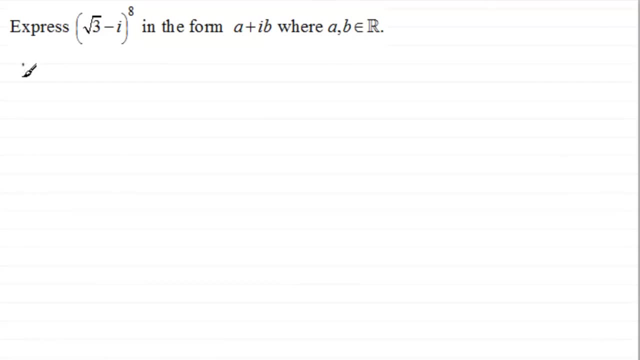 Let's just say we say that let z equal the complex number root 3 minus i. Now what I want to do is to work out what the modulus and the argument is, so I can represent z as a complex number in the mod-arg form. 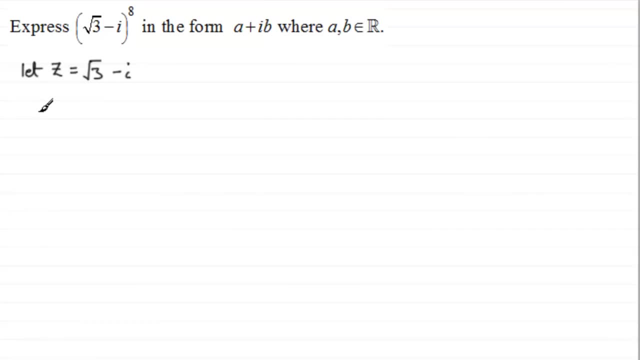 And to do this. what I'm going to do is just sketch an argon diagram. You might not want to do this. you might be able to just do it straight in your head, but I'll put it here just for reference, okay. 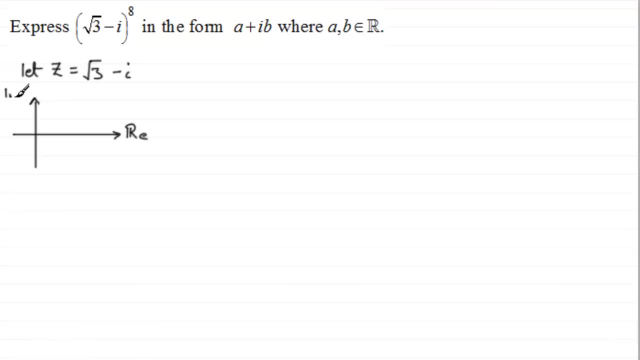 So we've got the real axis here and we've got the imaginary axis, And if we're looking at our complex number, z, root 3 minus i, it's going to be represented something like this: okay, So this is z, where we go. let's just mark this in: where we go, root 3 units to the right on the real axis and one unit down. 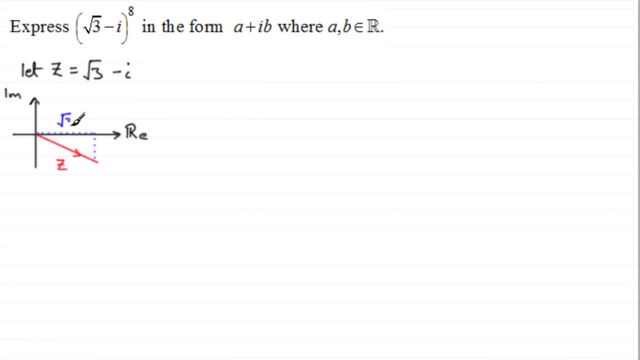 So if we just mark that in as being real, root 3 there and one unit down. so when it comes to working out the modulus of z, the length of this line, it's just done by Pythagoras's theorem. so we've got then that the modulus of z. 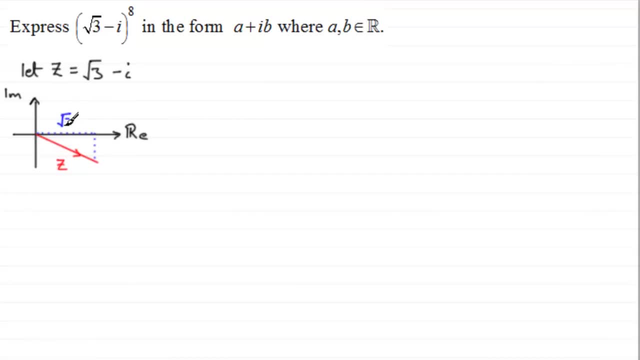 So if we just mark that in as being real, So we've got the real axis here and we've got the imaginary axis, root 3 there and one unit down. so when it comes to working out the modulus of z, the length of this- 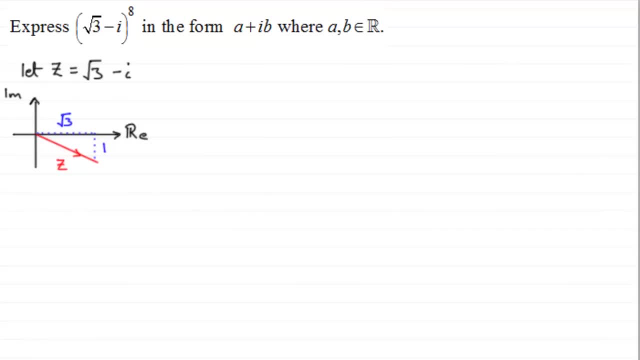 line. it's just done by Pythagoras's theorem. so we've got then that the modulus of z, okay, equals the square root then of the root of 3 squared root 3 squared plus 1 squared. in other words, we get 3 plus 1 is 4. root of 4 is 2. so there's the mod of z. 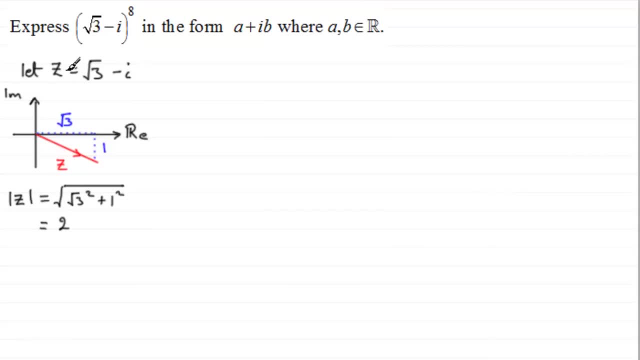 as for the arg of z, the arg of z is going to be this angle in here, okay, and it'll be written as a negative angle. remember, the arg of z must be an angle between minus pi and pi radians, so we've got to go in a clockwise direction here. well, first of all, we'll 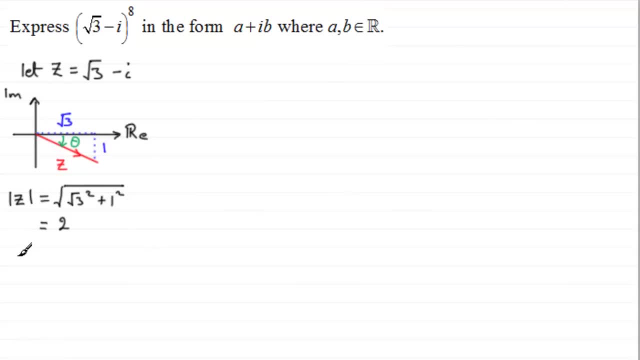 work out what this angle is, I'll call it theta. now theta would be equal to the inverse tan of the opposite side, which is 1 over the adjacent side root 3. so we've got the inverse tan of 1 over root 3, and if you work that out in your 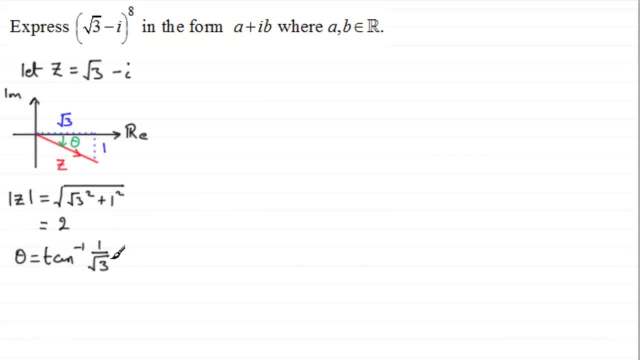 calculator. remember you need to work in radians mode. it is in fact pi upon 6. in degrees it would be 30 degrees, but in radians the exact value is pi upon 6 radians. so that means that therefore, the arg of z would be equal to minus pi upon 6. okay, so got to remember that. turning in this, 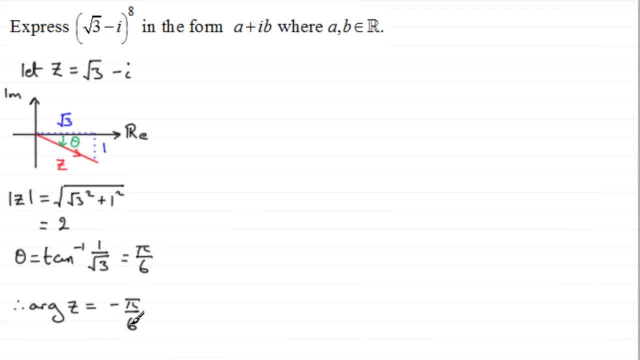 direction would be a negative turn minus pi upon 6 radians. okay, so having done that, we can now express this in mod-arg form. so what we have then is essentially that root 3 minus i okay to the power 8 can be expressed then in mod-arg form to the power 8. so you've got root 3 minus i is. 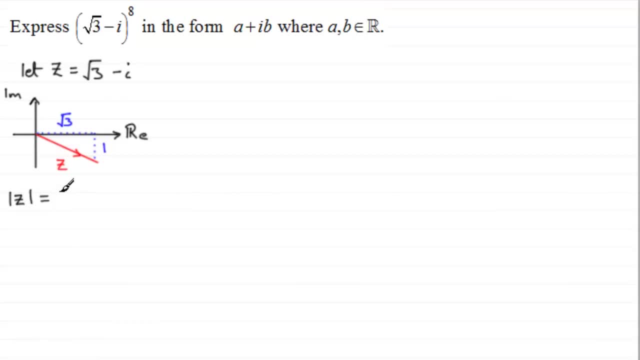 okay, equals the square root, then of the root of 3 squared root: 3 squared plus 1 squared. in other words, we get 3 plus 1 is 4. root of 4 is 2. so there's the mod of z. as for the arg of z, the arg of z is going to be this angle in here, okay, and it'll be. 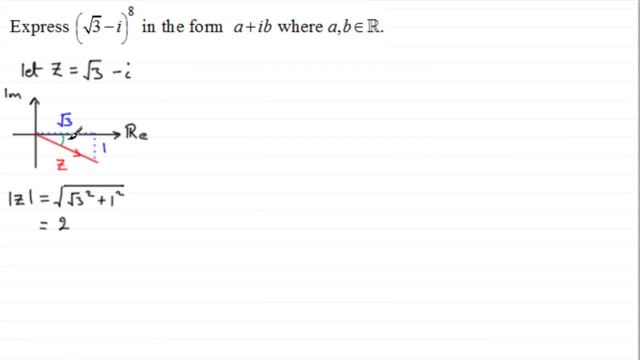 written as a negative angle. remember, the arg of z must be an angle between minus pi and pi radians, so we've got to go in a clockwise direction here. well, first of all we'll work out what this angle is. I'll call it theta. now, theta would be equal to the. 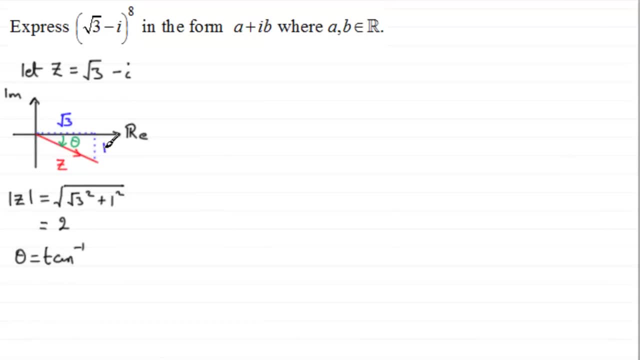 inverse tan of the opposite side, which is 1 over the adjacent side, root 3. so we've got the inverse tan of 1 over root 3. and if you work that out in your calculator, remember you need to work in radians mode. it is in fact pi upon 6. in degrees it would be 30 degrees, but in radians the 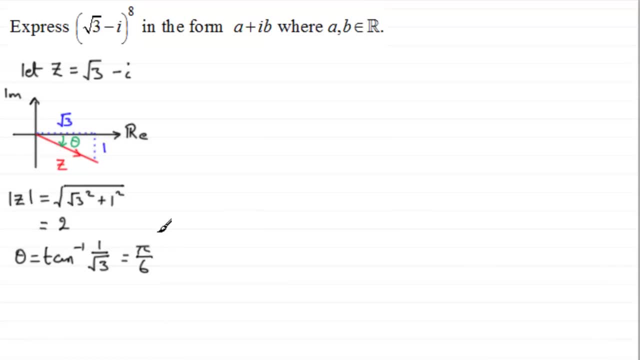 exact value is pi upon 6 radians. so that means that, therefore, the arg of z would be equal to minus pi upon 6. okay, so got to remember that turning in this direction would be a negative turn minus pi upon 6 radians. okay, so, having done that, we can now express this in mod-arg form. so what we? 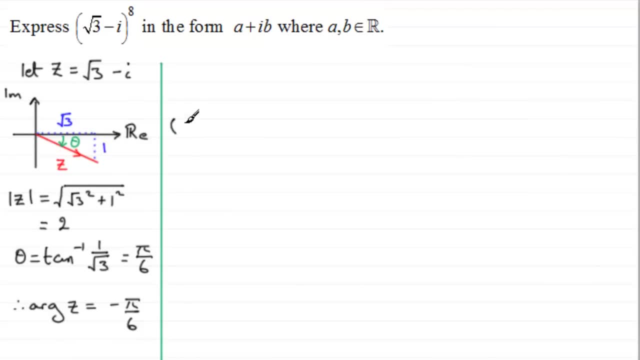 have then is essentially that root 3 minus i- okay to the power 8 can be expressed then in mod-arg form to the power 8. so you've got root 3 minus i is going to be 2, okay for the modulus 2, and then that's. 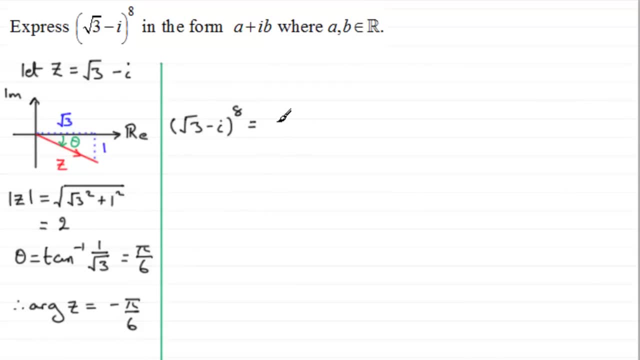 going to be 2. okay, for the modulus 2. and then that's going to be multiplied by the cosine of the arg, which is minus pi upon 6, and then plus i sine of minus pi upon 6, and then all of this- this, remember, is the mod-arg form for root 3 minus i. but all of this now. 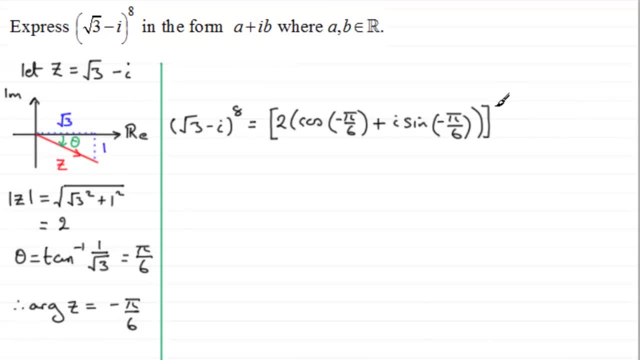 is raised to the power 8. okay, so we can expand this. we can rewrite this as: 2 to the power 8, and then the cos of minus pi upon 6, precise sine minus pi upon 6, all to the power 8. we'll do that here, so. 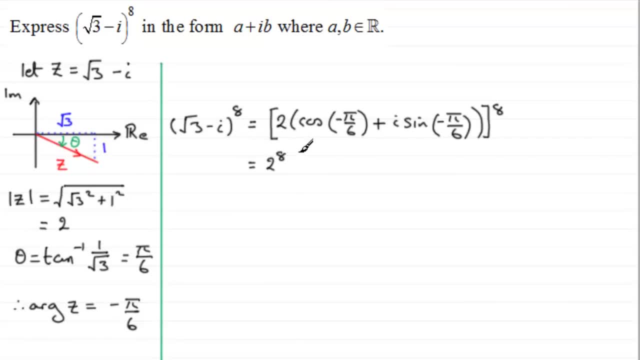 we've got 2 to the power 8, and then this is multiplied by the cosine of minus pi upon 6, plus i sine of minus pi upon 6, and all this is to the power 8. now, 2 to the power 8 is 256, so put that there. 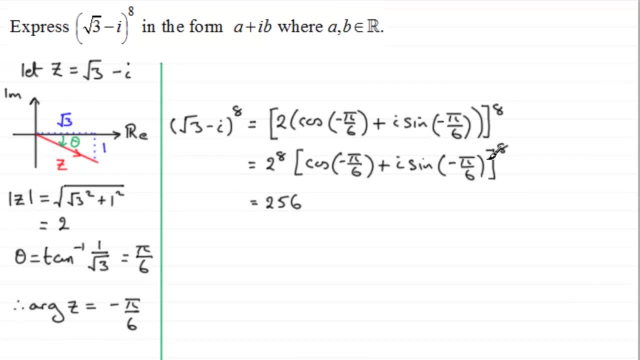 but when it comes to expanding this to the power 8, what we can do is now use de marva's theorem. so, And as a reminder, remember for DeMar's theorem, that is, if you've got z equals r, cos theta plus i sine theta. 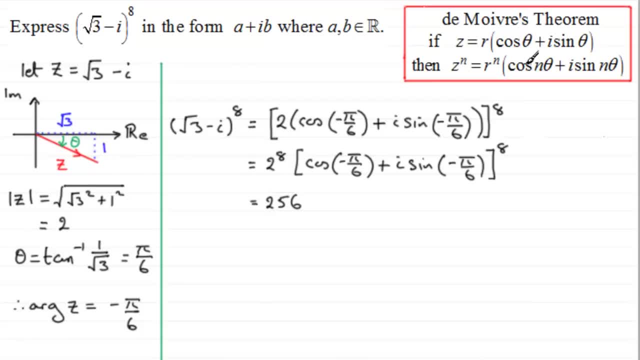 then z to the power n is equal to r to the power n, cos n theta plus i sine n theta. So what we can do is we can take our power and multiply it now by the arg. OK for the complex number here. So what we have then is that if we multiply the angle minus pi upon 6 by 8, we're going to get minus 8 sixths pi. 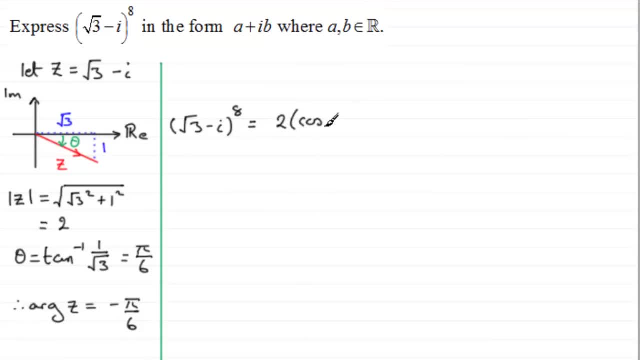 going to be multiplied by the cosine of the arg, which is minus pi upon 6, and then plus i sine of minus pi upon 6, and then all of this- this, remember, is the mod-arg form for root 3 minus i. but all of this now is raised to: 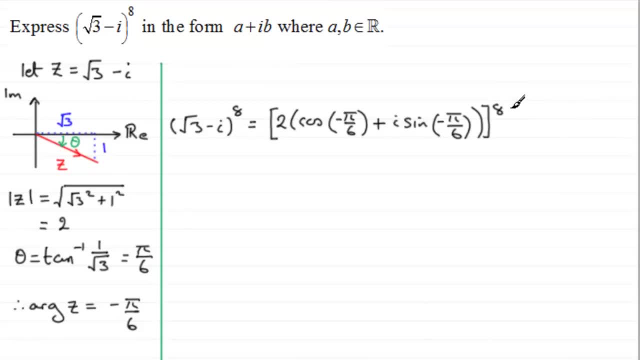 the power 8. okay, so we can expand this. we can rewrite this as 2 to the power 8 and then the cos of minus pi upon 6, precise sine minus pi upon 6, all to the power 8. we'll do that here. so we've got 2 to the power 8 and then this is multiplied by the cosine of minus. 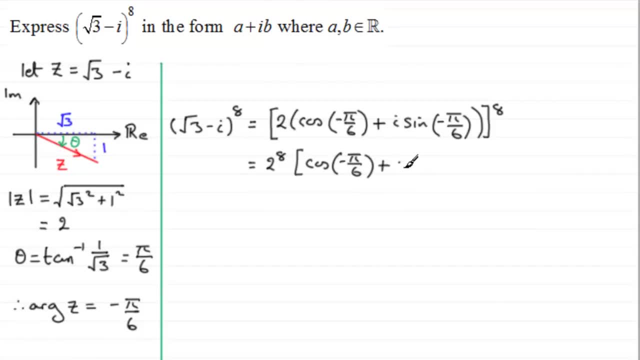 pi upon 6 plus i sine of minus pi upon 6, and all this is to the power 8. now, 2 to the power 8 is 256, so put that there. but when it comes to expanding this to the power 8, what we can, 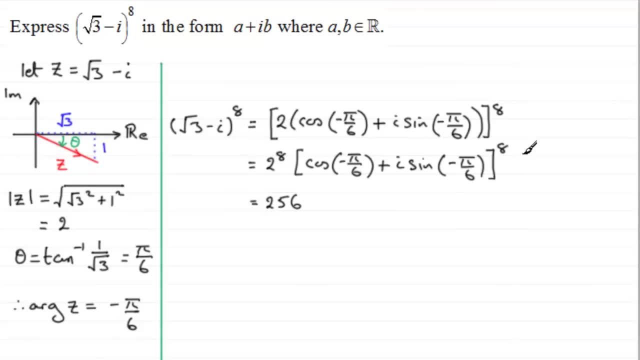 do is now use de marva's equation, De Marva's theorem and, as a reminder, remember for de marva's theorem, that is, if you've got z equals r cos theta plus i sine theta, then z to the power, n is equal to r to the power. 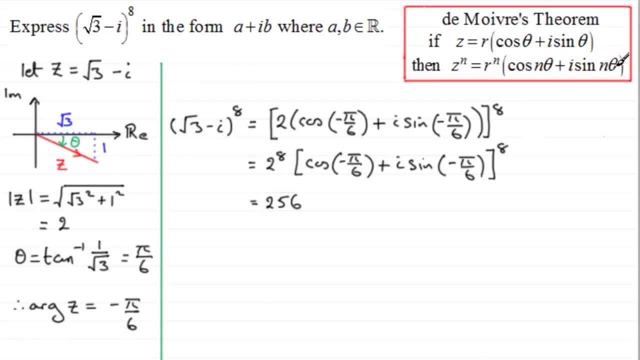 n cos n theta plus i sine n theta. so what we can do is we can take our power and multiply it now by the arg. okay for the complex number here. So what we have then Is that if we multiply the angle minus pi upon 6 by 8, we're going to get minus 8 sixths. 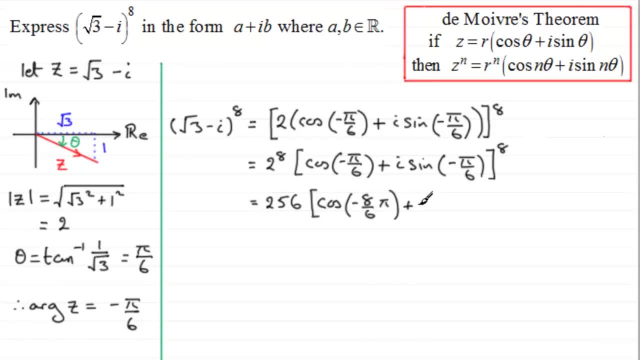 pi. okay, and the same with the sine- here i sine- of minus 8. pi over 6. okay, so that's applying de marva's theorem. let's just put an arrow to that, okay, to signify that. Now what we've got next is that this is equal to 256. but when we're working out the cosine, 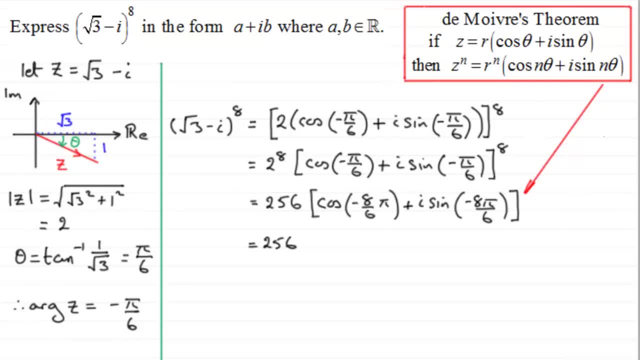 of minus 8 sixths pi, which really reduces down to 4 thirds. we'll just cancel that out. there 4 thirds and 4 thirds there. okay, so it's a minus 4 thirds pi when we're doing this, So we can enter that, I suppose, straight into your calculator, or, being a fairly standard. 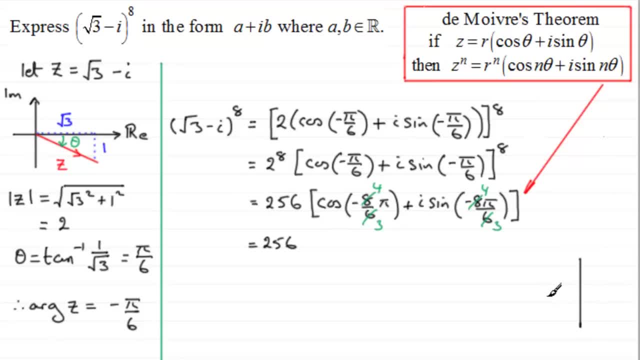 result. you might want to just think of the quadrants- okay, we'll just do it here- where this is 0 radians and a turn of minus 8 sixths pi or minus 4 thirds pi is going to take you in a clockwise sense to this quadrant round here. 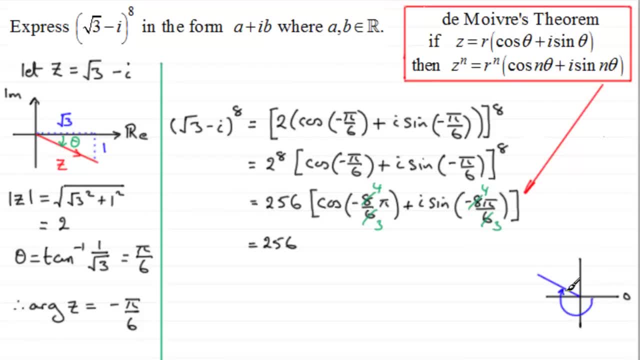 This Is going to represent a turn of minus 8 sixths pi or minus 4 thirds pi, so it's exactly the same as working out a turn in this direction, which would be 2 thirds pi. okay, so you could argue whether you want to keep it like that or whether you want to change it. it's up to. 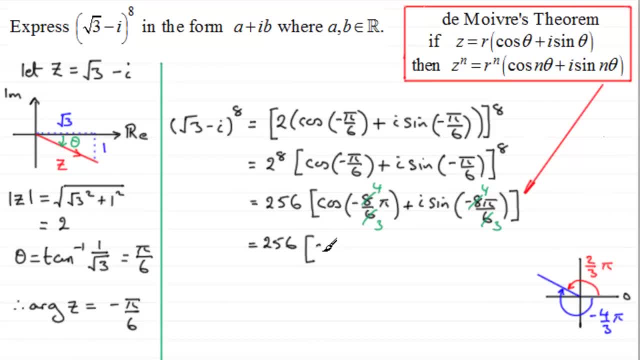 you. You could rewrite this as the cosine of minus 8 sixths pi. You could rewrite this as the cosine, then, of 2 thirds pi. okay, plus i sine of 2 thirds pi. Right, and then, if you work out these values, the cosine of 2 thirds pi is minus a half. 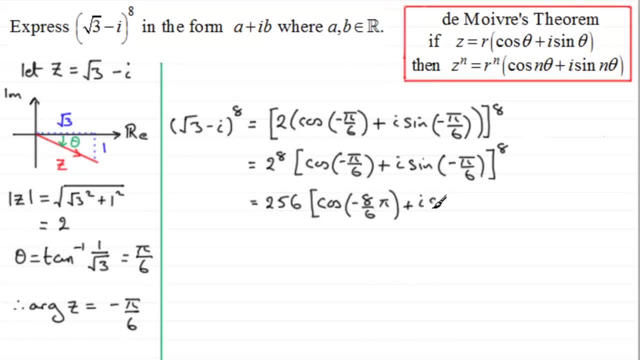 OK, and the same with the sine- here i sine- of minus 8 pi over 6.. OK, so that's applying DeMarva's theorem. Let's just put an arrow to that, OK, to signify that. Now. what we've got next is that this is equal to 256.. 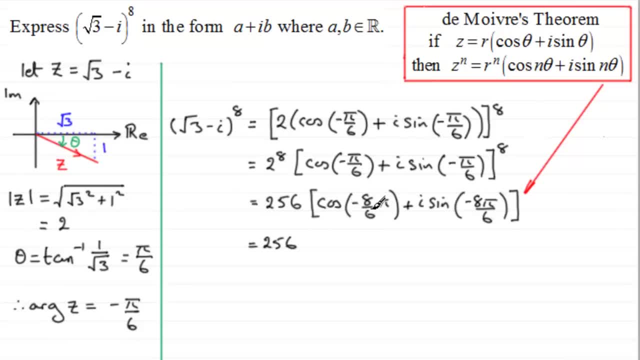 But when we're working out the cosine of minus 8 sixths pi, which really reduces down to four thirds, we just cancel that out. there. four thirds and four thirds there, OK. so it's a minus four thirds pi, OK. 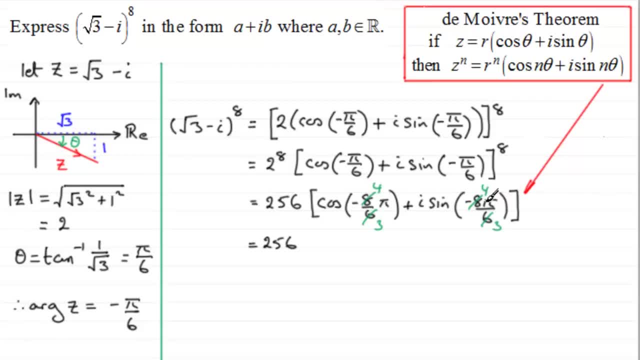 When we're doing this. you could enter that, I suppose, straight into your calculator or, being a fairly standard result, you might want to just think of the quadrants- OK, we'll just do it here- where this is zero radians and a turn of minus 8 sixths pi or minus four thirds pi is going to take you in a clockwise sense. 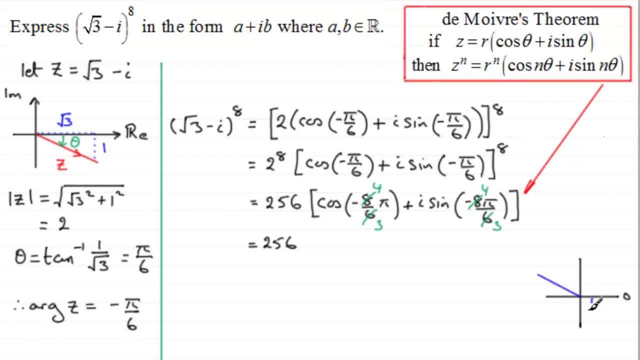 to this quadrant round here. This would represent a turn of minus 8 sixths pi or minus four thirds pi. So it's exactly the same as working out a turn in this direction, which would be two thirds pi. OK, so you could argue whether you want to keep it like that or whether you want to change it. it's up to you. 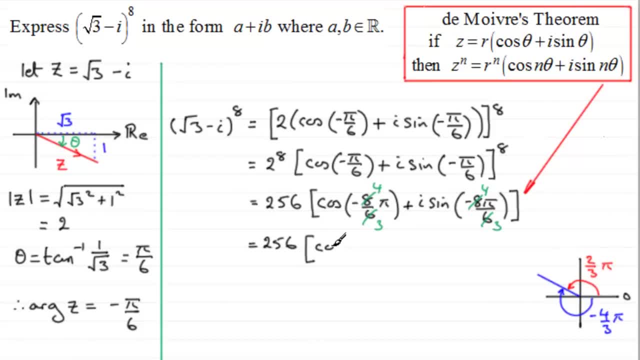 You could rewrite this. So you could rewrite this as the cosine then, of two thirds pi, OK, plus i sine of two thirds pi, Right. And then, if you work out these values, the cosine of two thirds pi is minus a half. 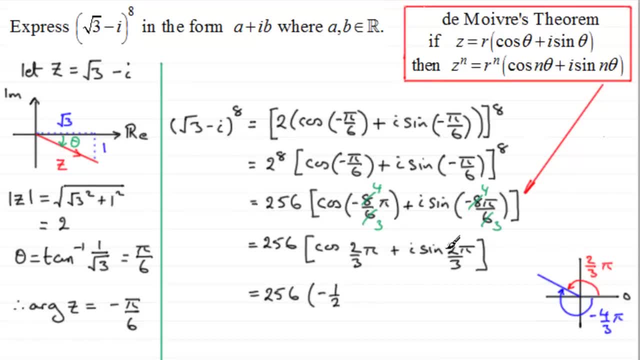 So you've got minus a half and then for the sine of 2 thirds pi, that is root 3 over 2. so you multiply by the I and you've got plus I root 3 over 2. and if we multiply each of these two,